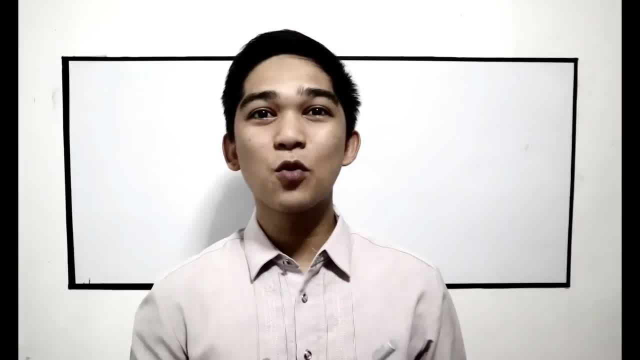 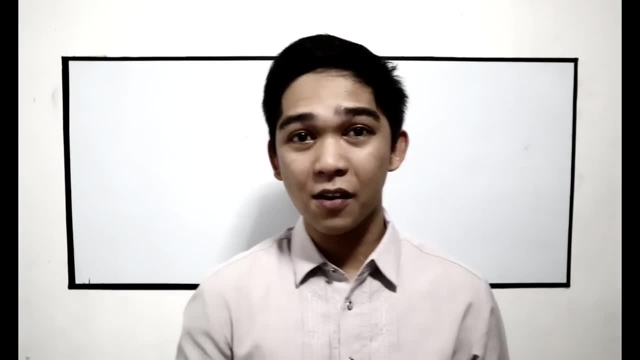 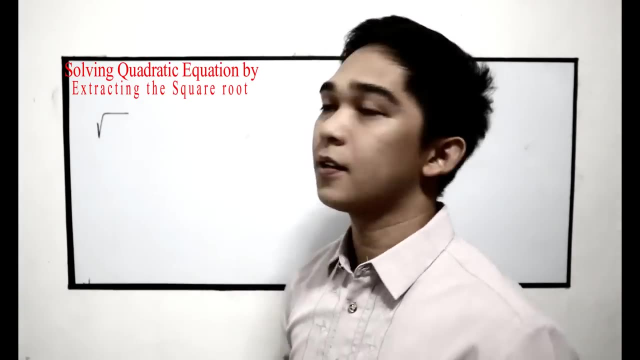 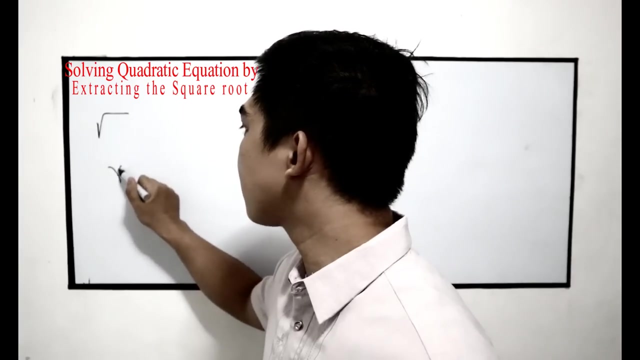 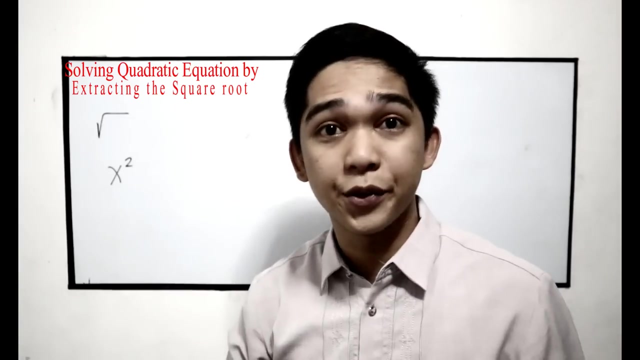 Welcome to lesson one, Solving quadratic equation by extracting the square root From our topic itself. we have the square root And this is the symbol for square root. That symbol, Let's say, if we have x square, What is the relationship of the square and the square root? 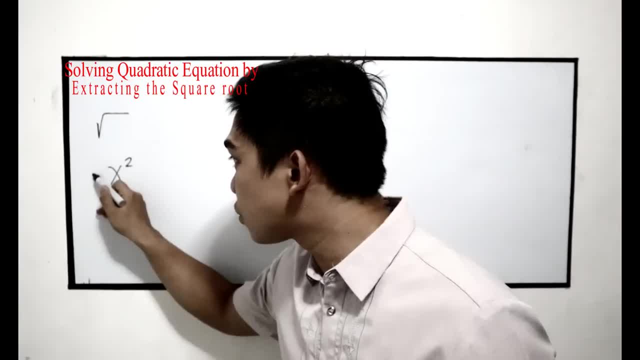 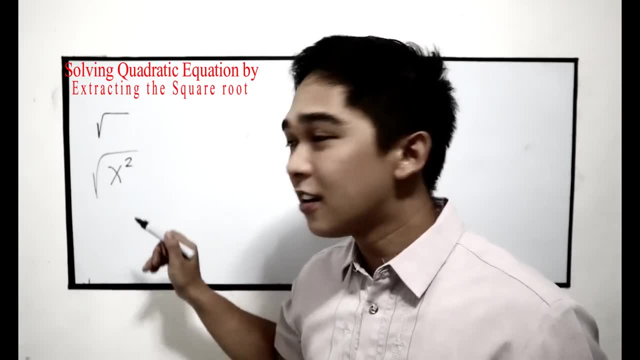 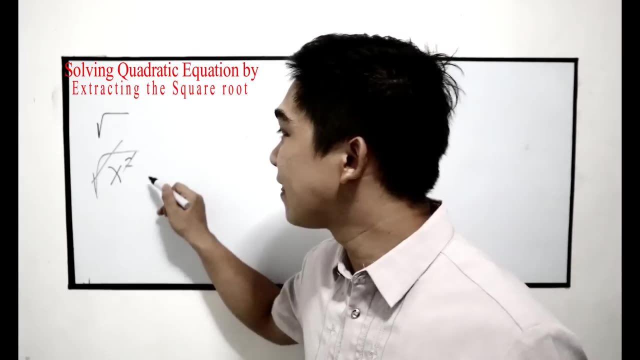 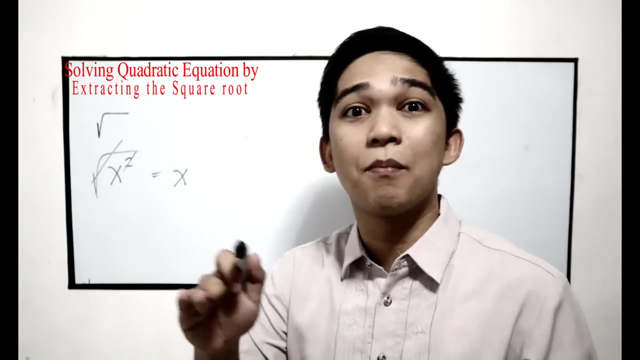 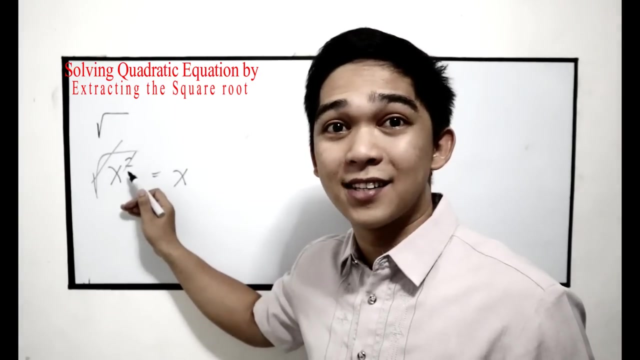 In this expression. if we're going to extract the square root, the relationship will be: square root will be cancelled out and this square will be cancelled out, And this will become equal to x, Applying your previous lesson about the laws of exponent. why is the square root? and square will be cancelled out. 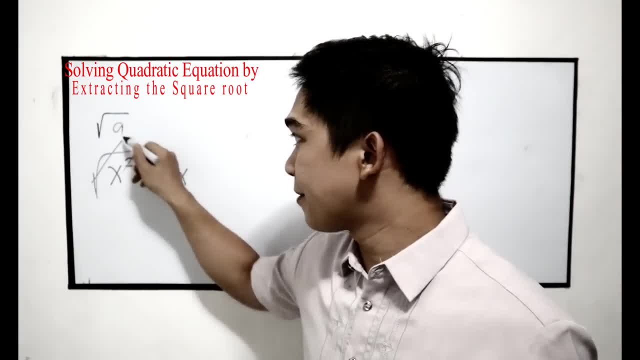 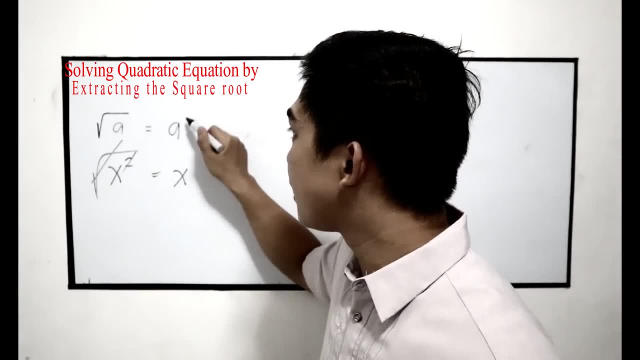 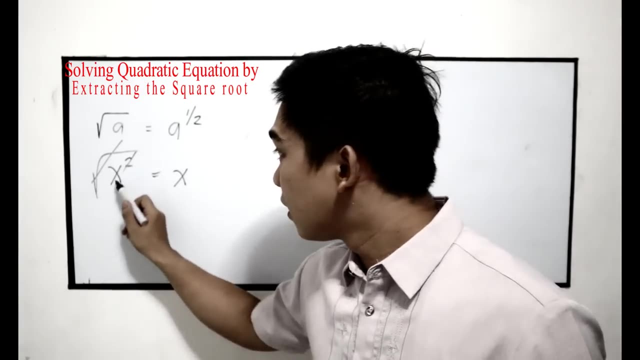 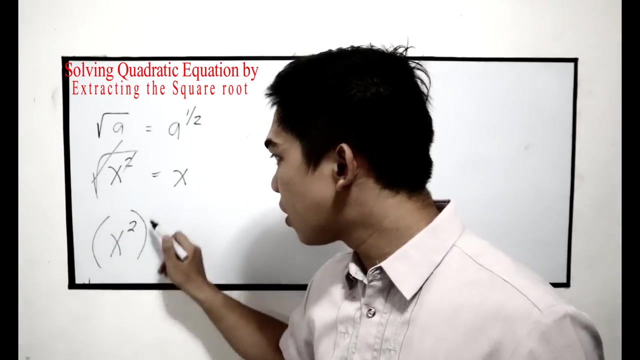 Let's say the square root of a. We know that the equivalent of square root of a is a raised to 1 half. Applying this, one x squared and the value of square root is 1 half. So we need 2 raised to 1 half. 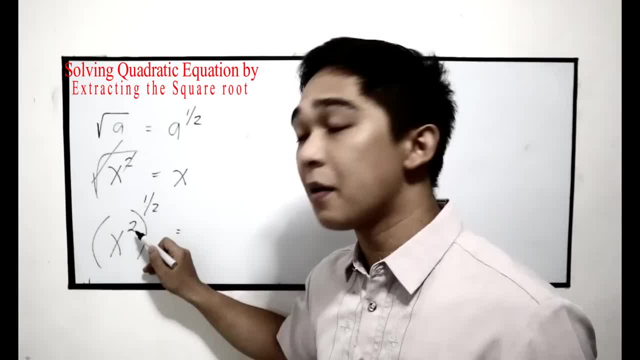 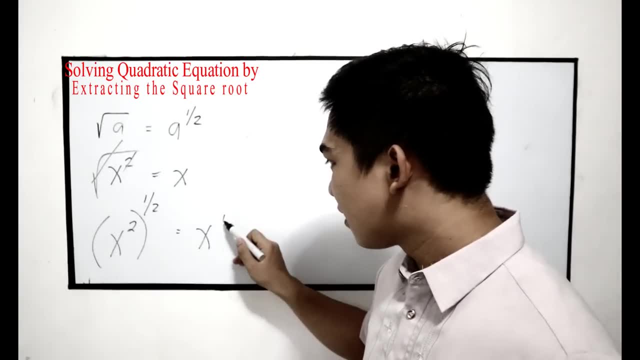 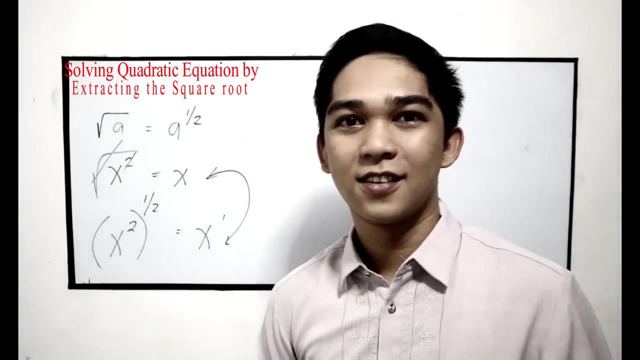 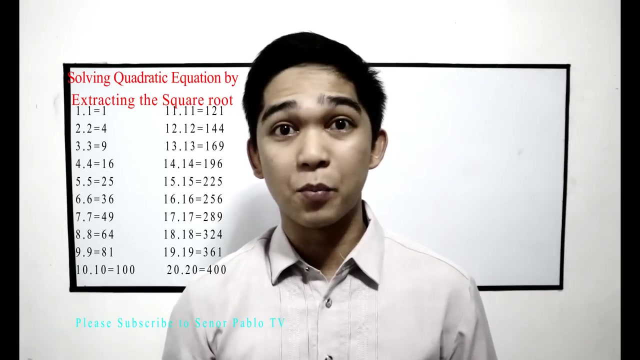 Power to a power 1 half times 2. That is equivalent to 1.. That means x raised to 1 is also equal to x. Again, press f to get 1 half of the value of square root and then y raised to 1 half. 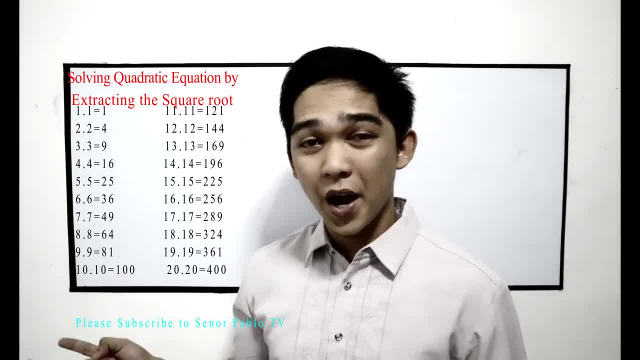 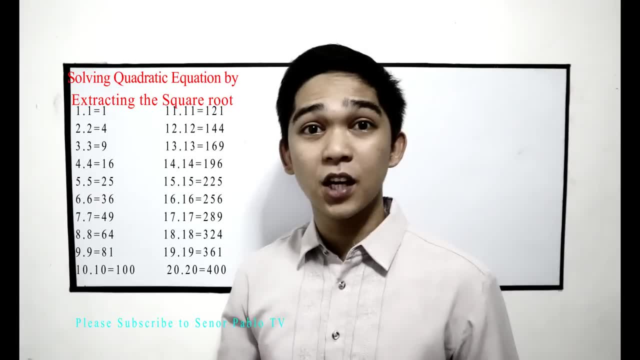 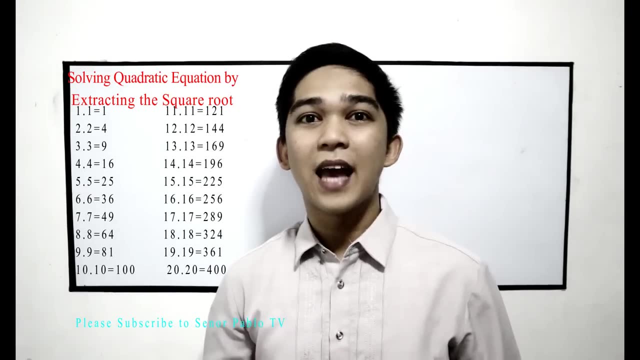 In this lesson it is very important that you are familiar with the perfect square numbers. First let us recall If you have 1 squared, or 1 x 1. which is nine four square four square, which is four times four, is equal to 16.. 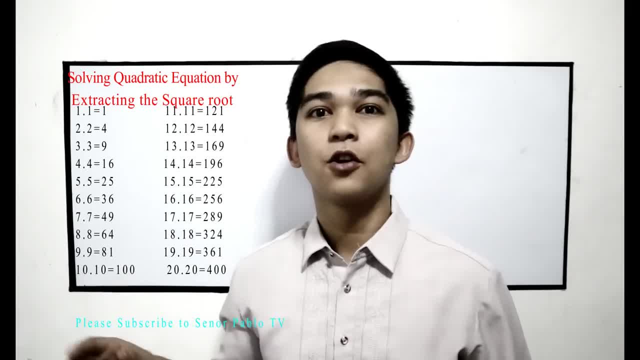 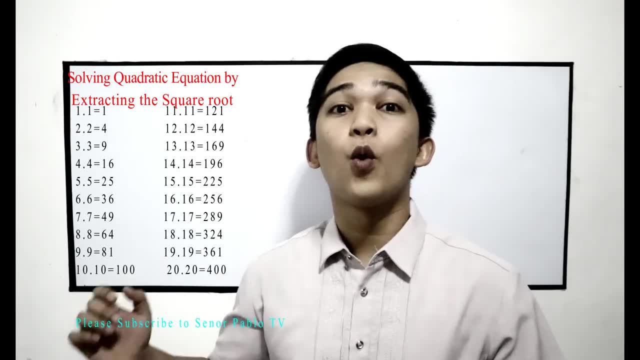 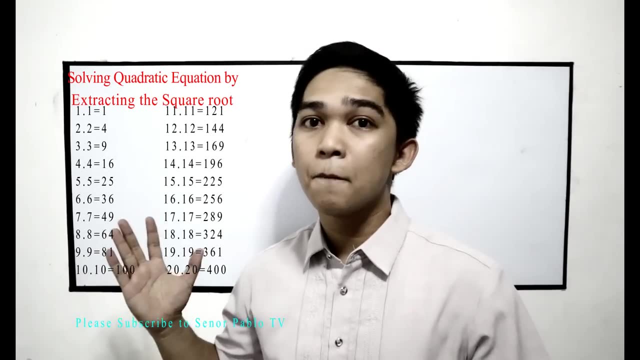 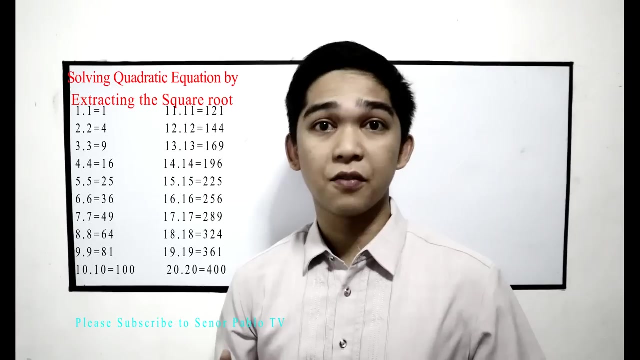 and we have 25, 36, 49, 64, 81, 100, 121, 144 and so on. so in order for you to solve, extracting the square root easily, you need to memorize those or at least familiarize. let us proceed in solving number one. 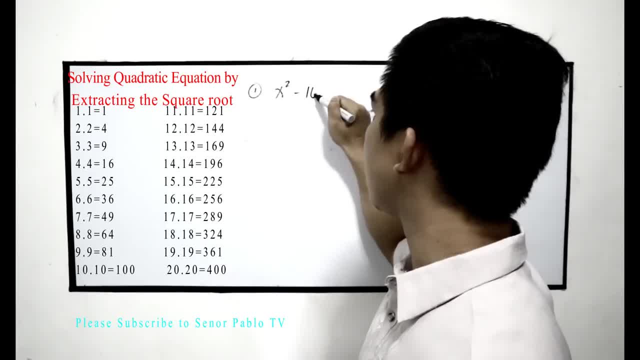 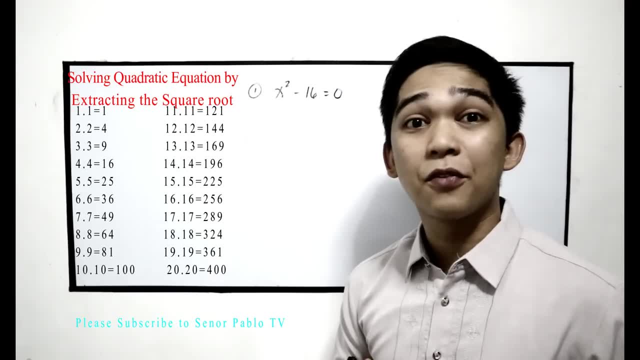 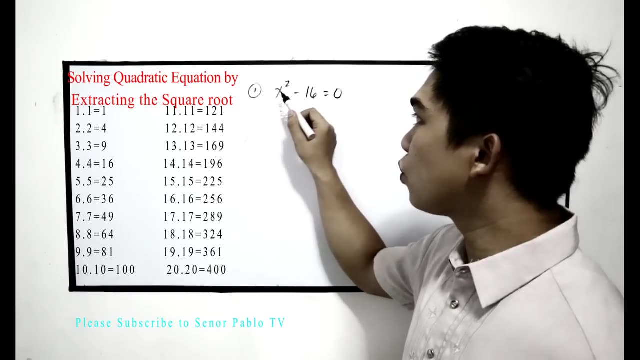 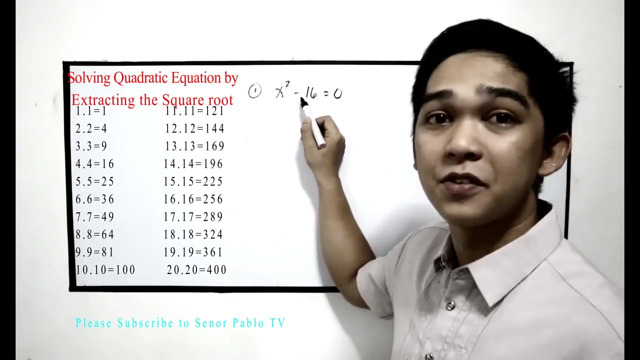 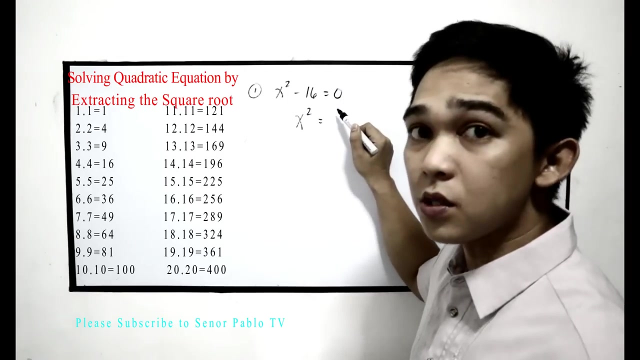 let's say x squared minus 16 is equal to zero. solve by extracting the square root. we need to find the value for x. in this case we need to isolate our variable. that means we need to transpose negative 16.. so x square is equal to negative. transpose that will become: 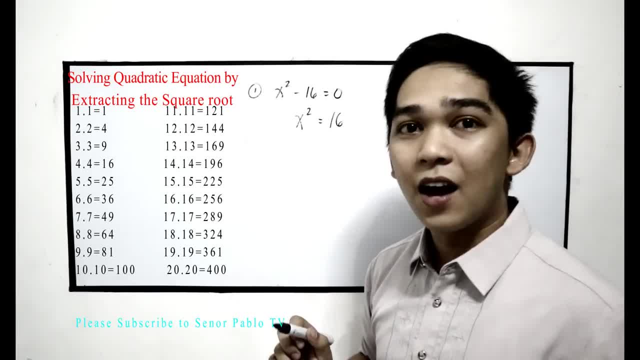 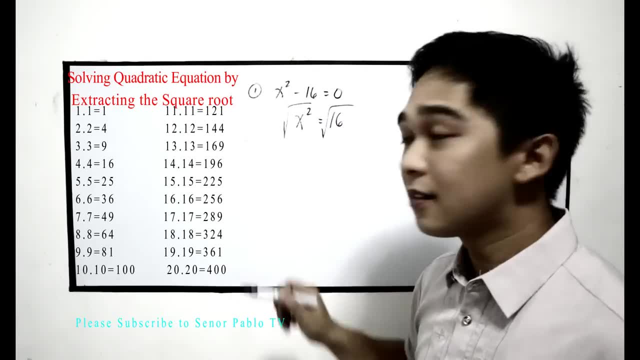 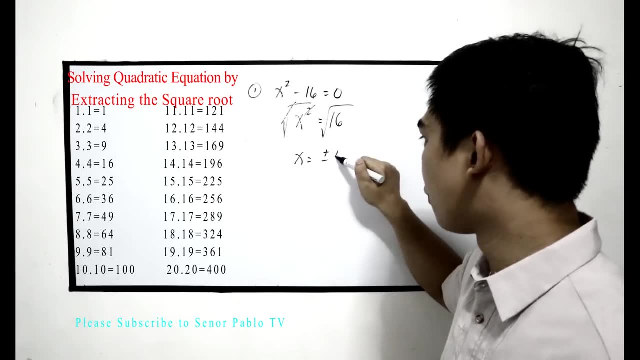 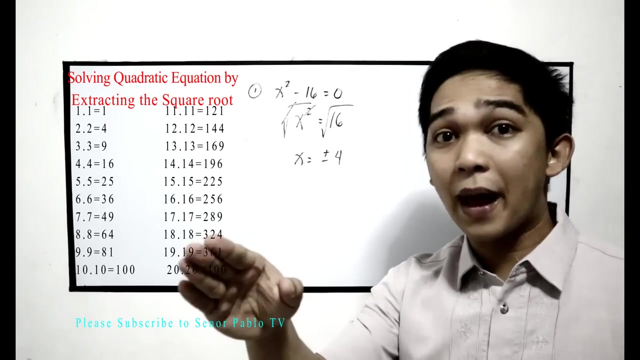 positive, 16.. now get the square root. square root, square root. so this will be cancelled out. now x is equal to positive, negative, 4.. why we need to have the positive and negative sign? because we have 4 positive, 4 times positive, 4. 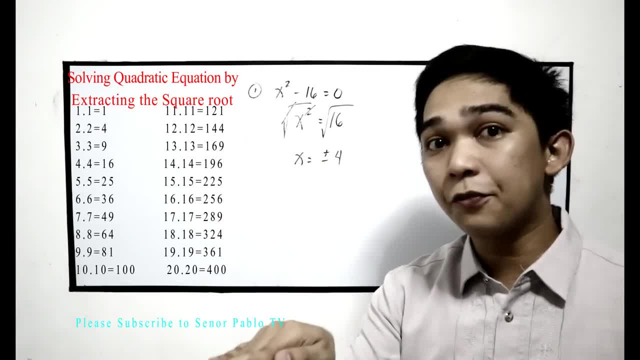 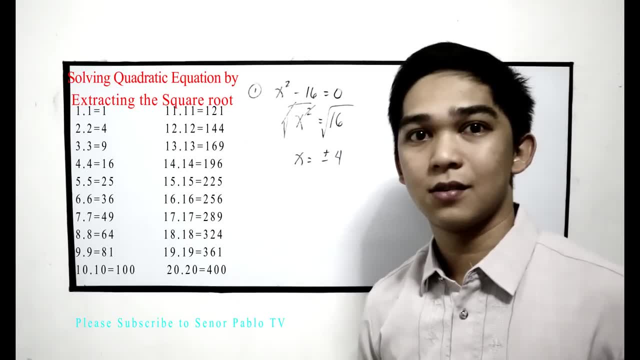 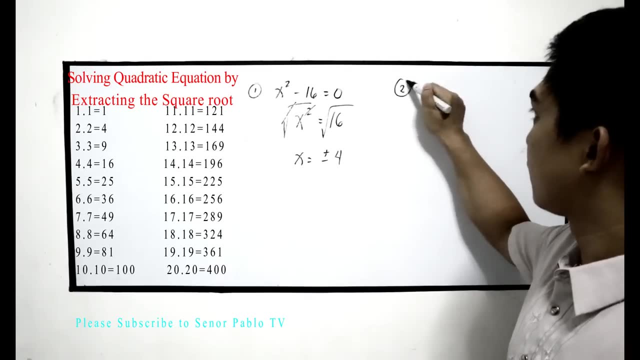 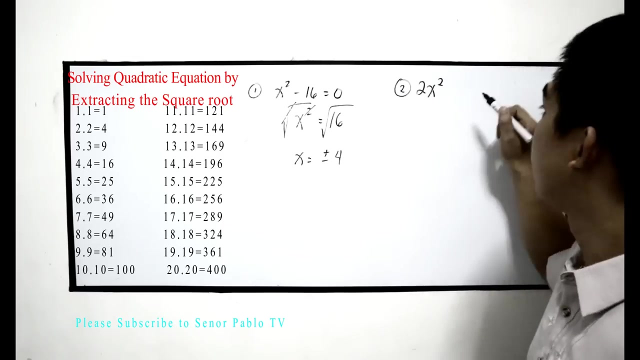 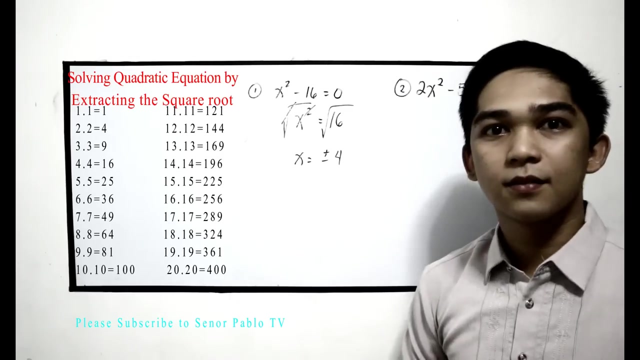 that is 16.. the other one is negative 4 times negative. 4 is also positive 16. so we have two solutions: the positive 4 and the negative 4.. another one is: 2x squared minus 50 is equal to 0.. 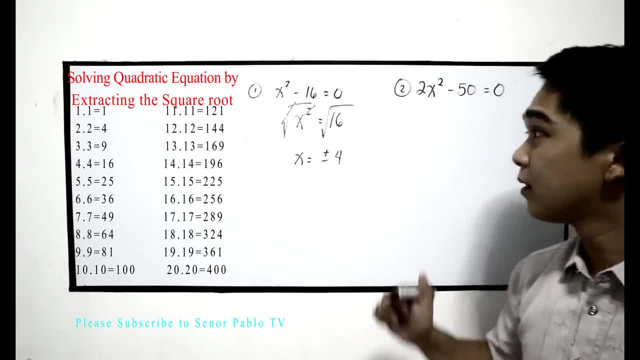 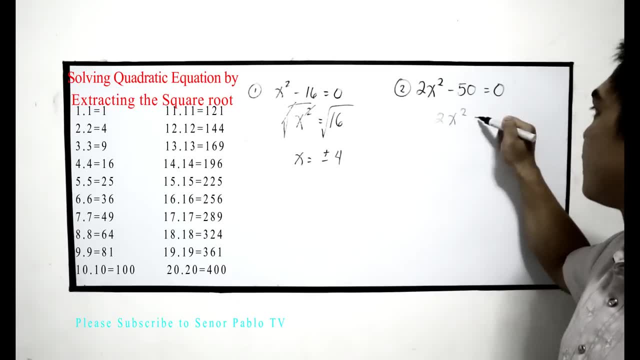 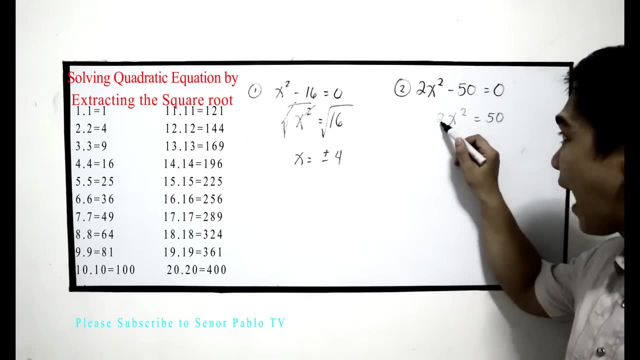 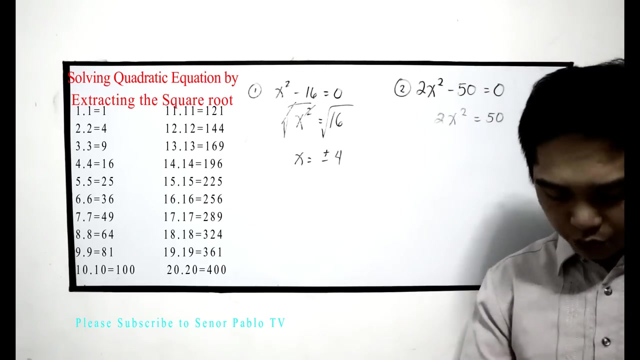 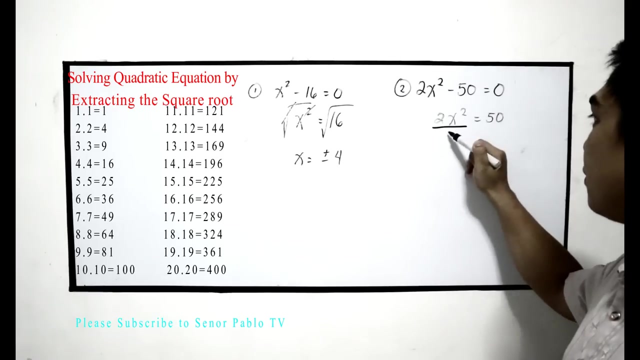 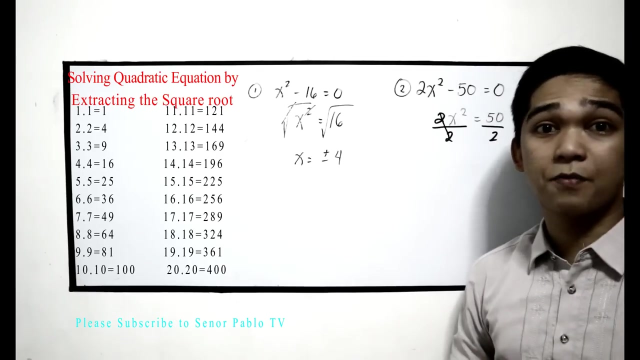 again isolate your variable. so transpose to 2x squared is equal to 2x squared minus 50- 50. Now we have coefficient 2.. We need to remove the coefficient 2.. So we need to divide by 2.. Divided by 2, this will be cancelled out because 2 divided by 2 is 1.. 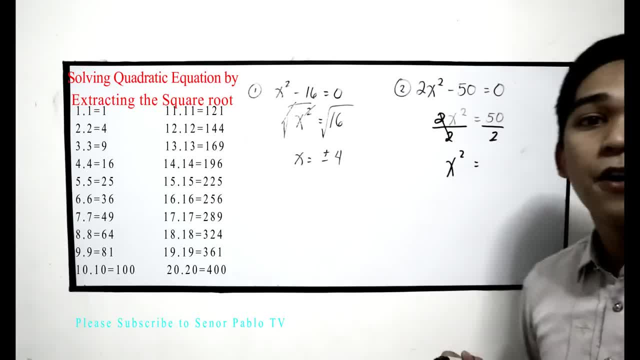 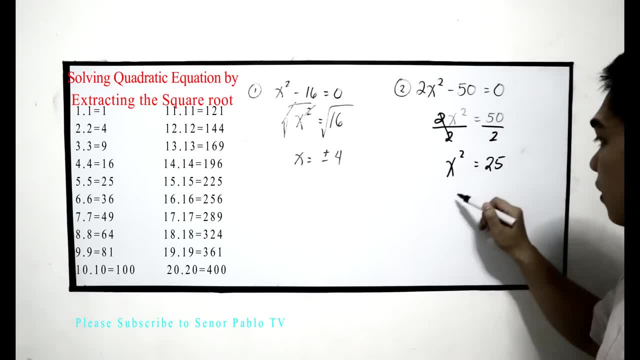 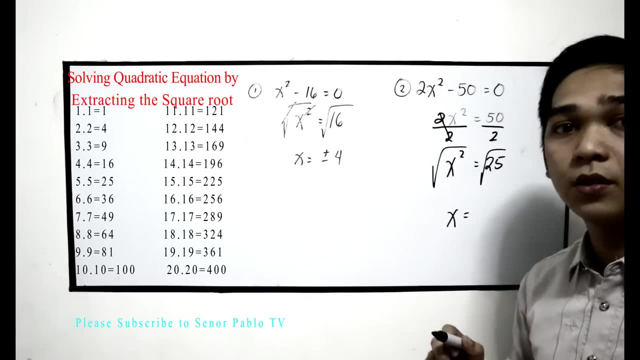 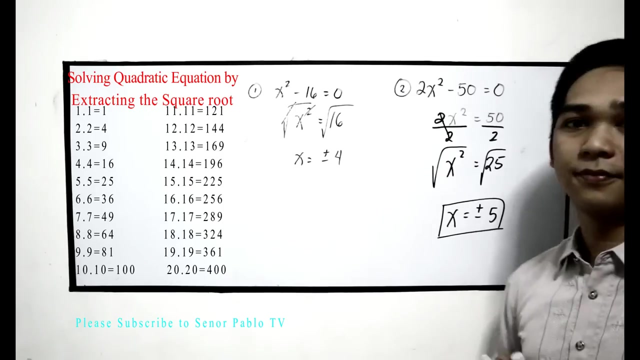 Therefore we have: x squared is equal to 50 divided by 2. That is 25.. Extract the square root, So x is equal to the square root of 25, is positive, negative, 5.. Another example, number 3.. 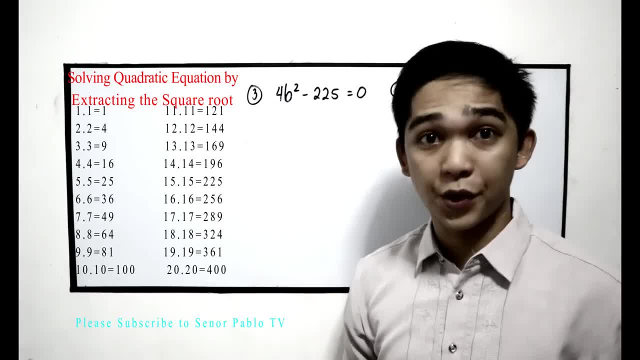 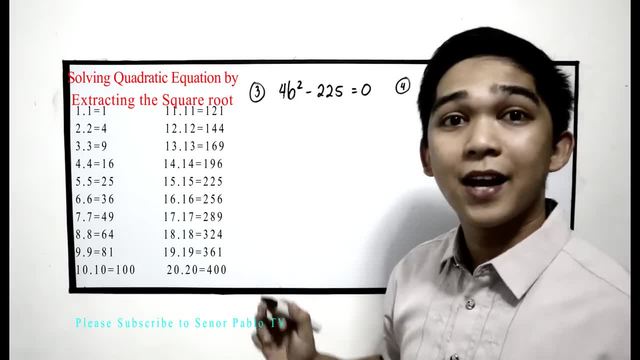 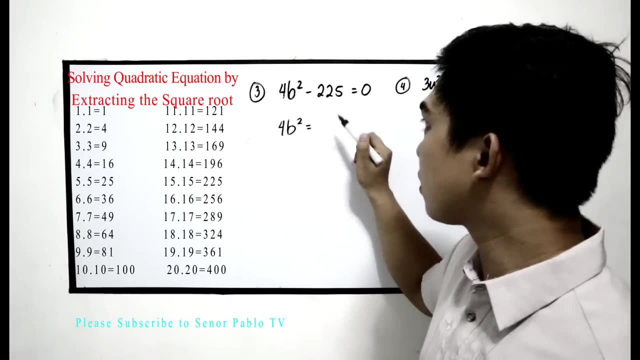 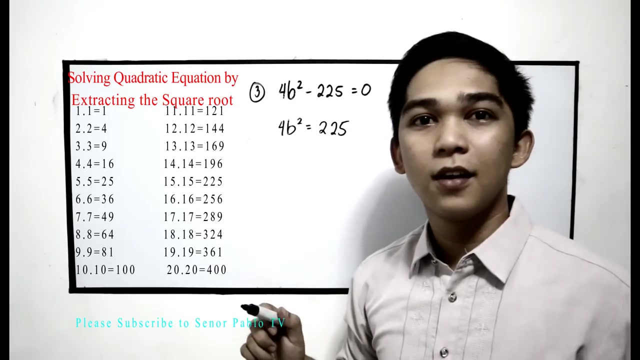 4b squared minus 225 is equal to 0.. The same step: isolate the variable, So we need to transpose negative 225.. So the remaining is 4b squared happy is equal to transpose 225 positive 225.. 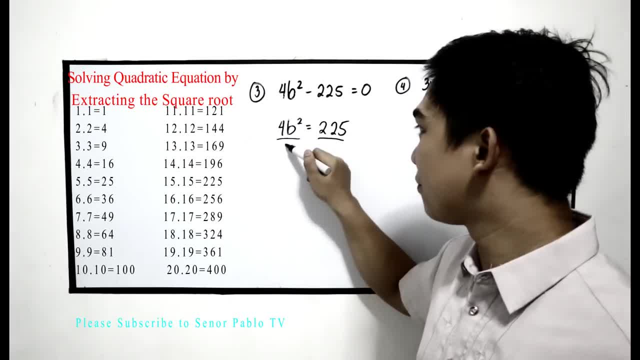 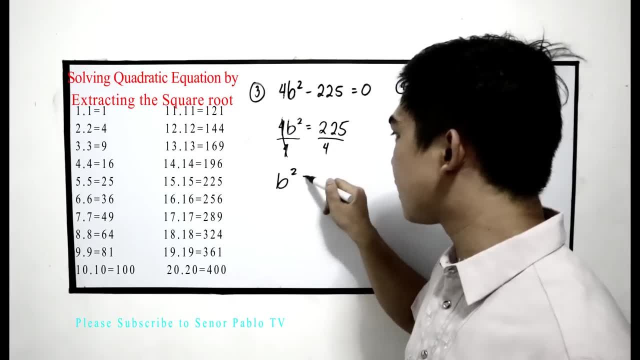 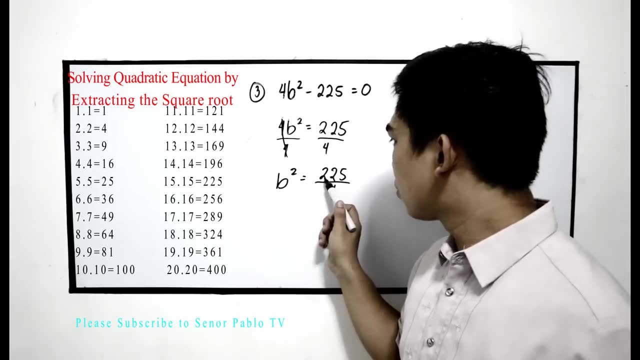 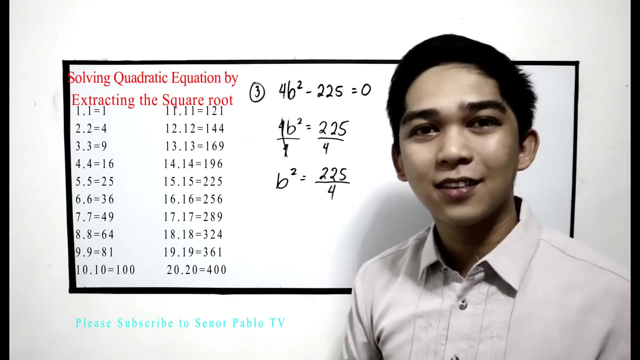 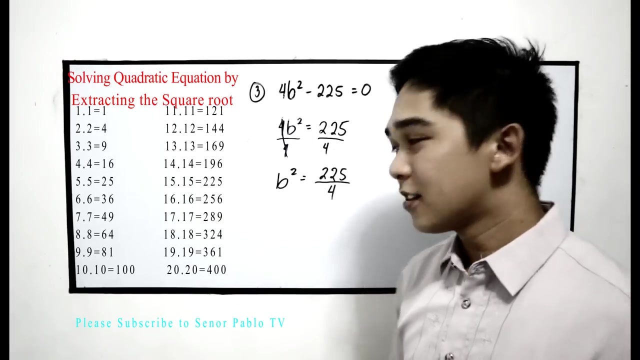 Now divide by 4.. The remaining will be b squared is equal to 225 over 4.. 225 divided by 4.. Is it divisible? No, But notice that 225 and 4 are perfect square number, So that means we need now to multiply. 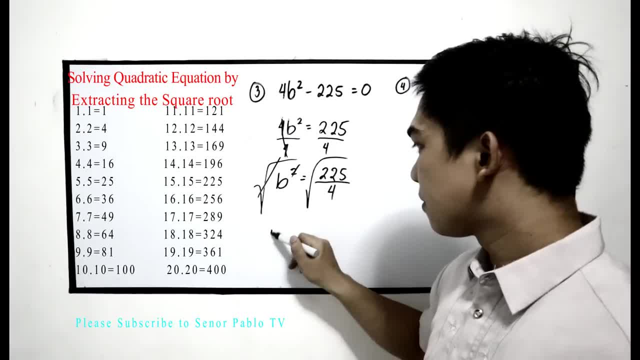 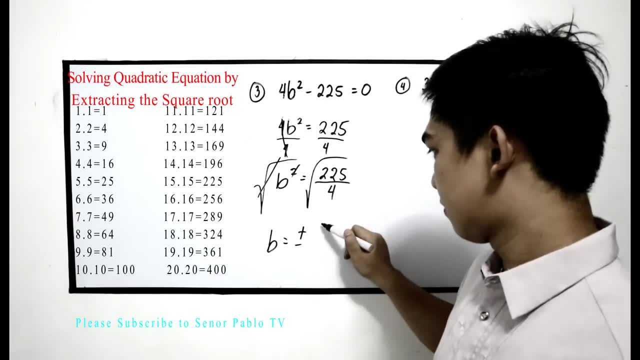 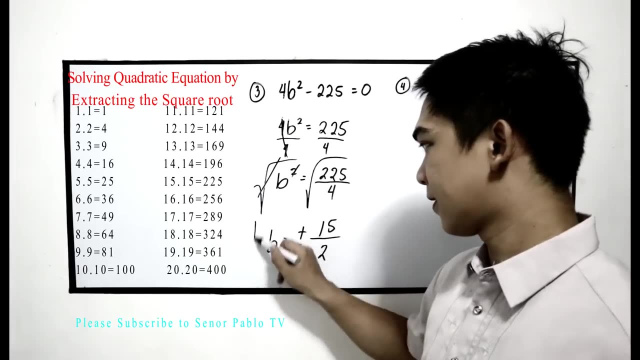 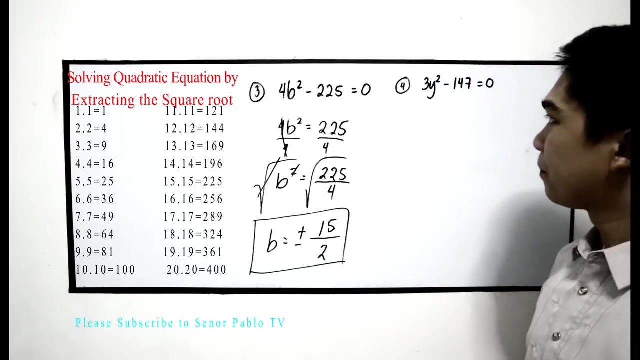 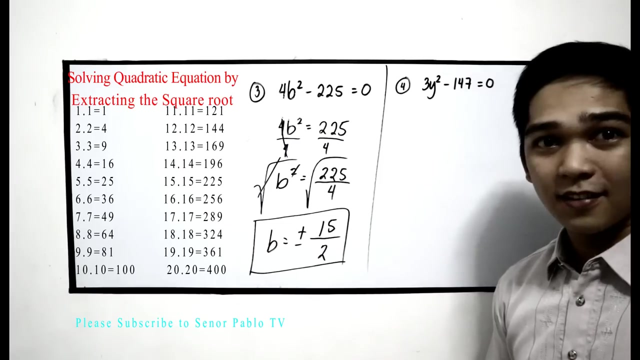 to extract the square root b is equal to positive, negative square root of 225, that is 15, over square root of 4, that is 2.. This is now our final answer. For example, 3y squared minus 147.. The same process: isolate the variable. Copy 3y. 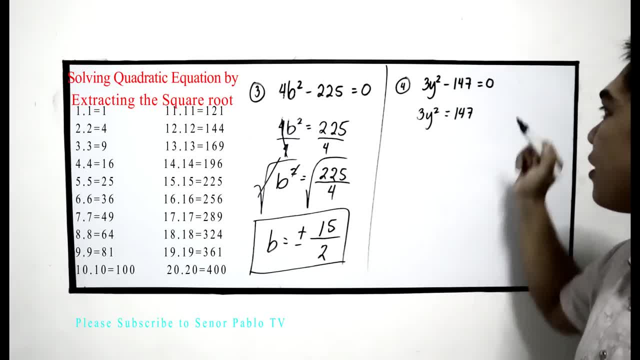 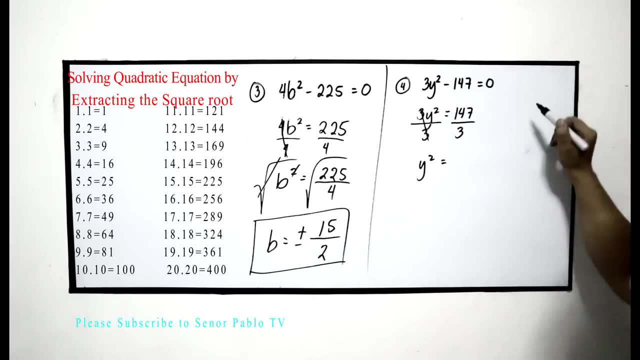 squared is equal to 147.. Now divided by 3.. Y squared is equal to 147 divided by 3.. So let us divide 14 divided by 3, that is 4, 4 times 3, 12,. then subtract 14 minus 12, 2, bring it down: 7, 27 divided by 3, that is 9.. 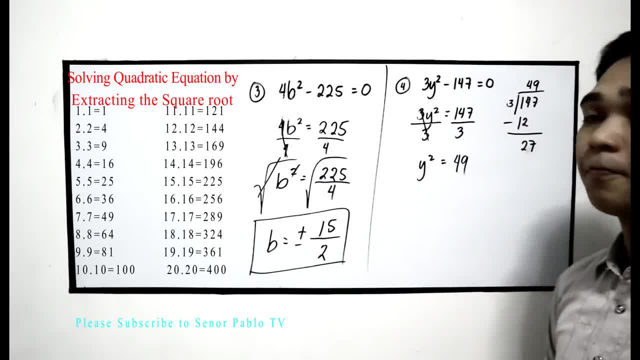 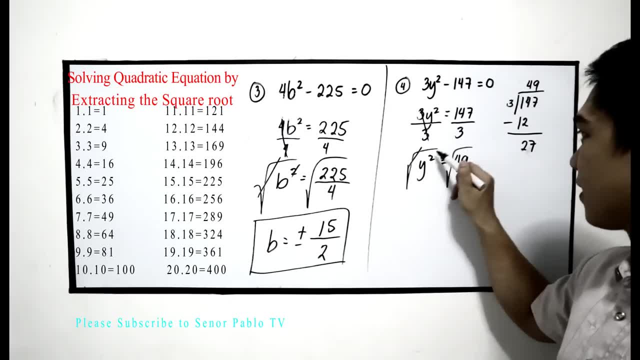 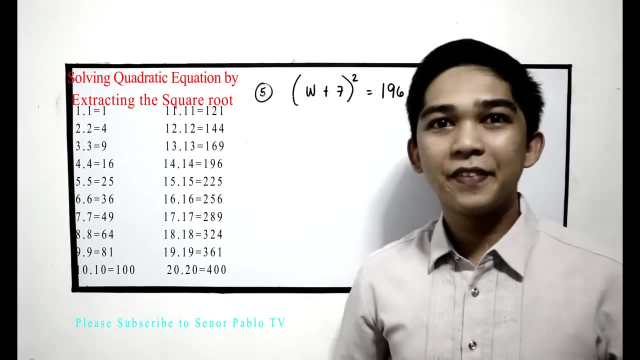 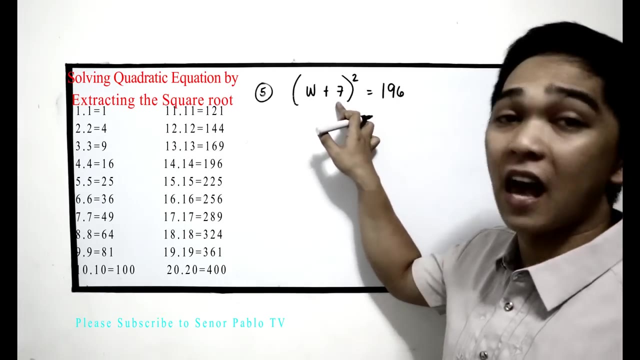 So we now have 49.. To find y, get the square root. y is equal to positive, negative, 7.. And now our last example, number 5.. Quantity w plus 7 raised to 2 is equal to 196..